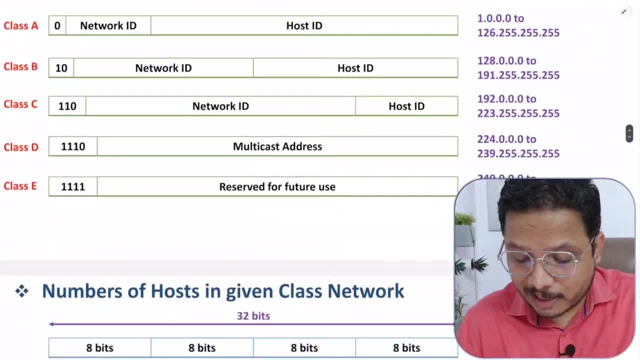 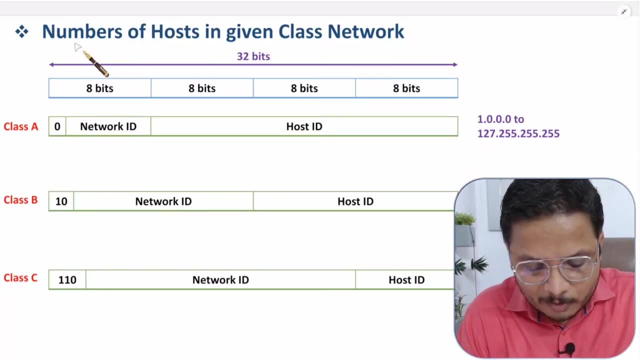 all those classes are defined and how we can identify which IP address belongs to which class. After that I'll explain you some interesting fundamentals in which I'll explain you how many number of posts that is given in this given class of network And along with that, 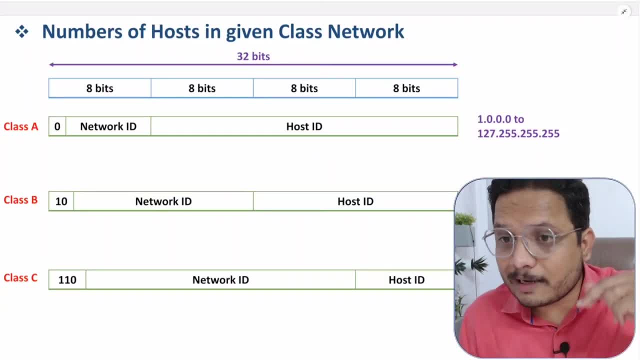 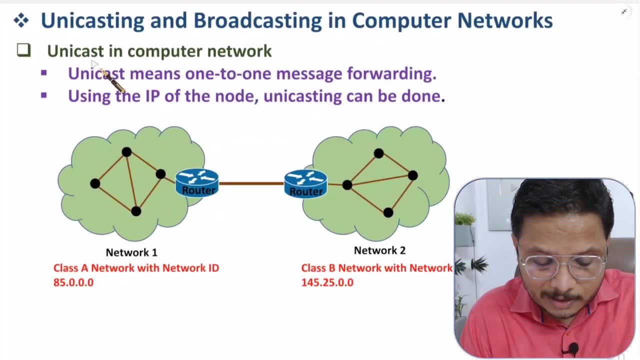 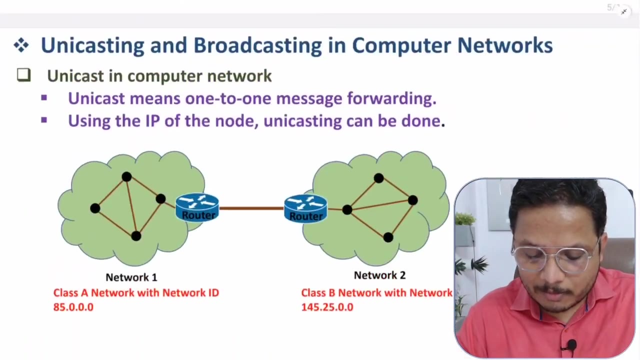 I'll explain you how we can have network IP And for that network IP what will be broadcast IP address. And then I'll explain you how we can have unicasting and broadcasting, And that I'll explain you by practical examples. So let us see first how many basics are there with IP addresses. So in basics of IP addresses, 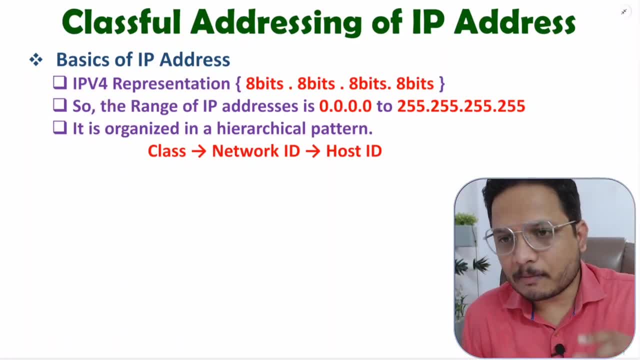 I'll be discussing about IPv4 addresses Here. basically, two types of IP addresses are there. One is IPv4. And second is IPv6.. I'll be discussing about IPv4 addresses in this video. See in IPv4 representation. it is having size of 3.5.. 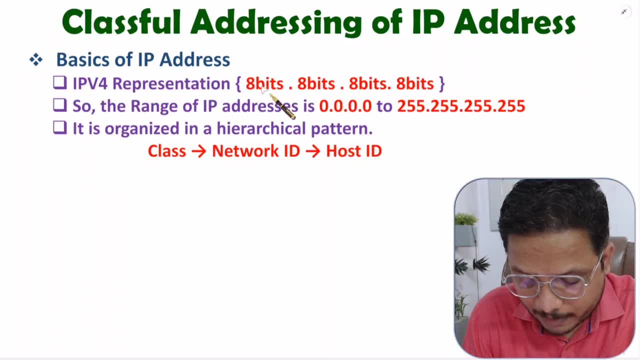 It is represented as per 8 bits: dot 8 bits, dot 8 bits, dot 8 bits. 8 bits means 1 byte, or you can say 1 octave, So 4 octaves are there And that representation as per octave. 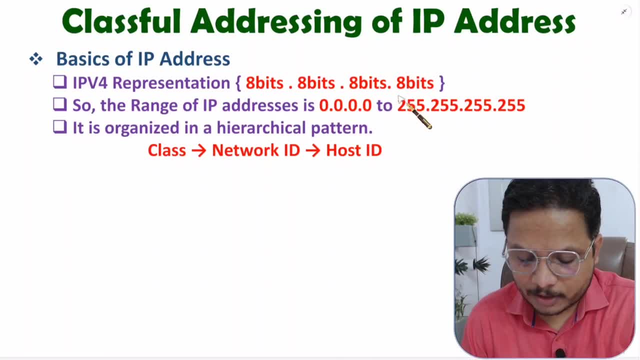 dot octave, dot octave, dot octave. That is how it is And you should know 8 bits is having how much size. 2 to the power, 8 means 256.. So it is having range from 0 to 255.. 256 means: 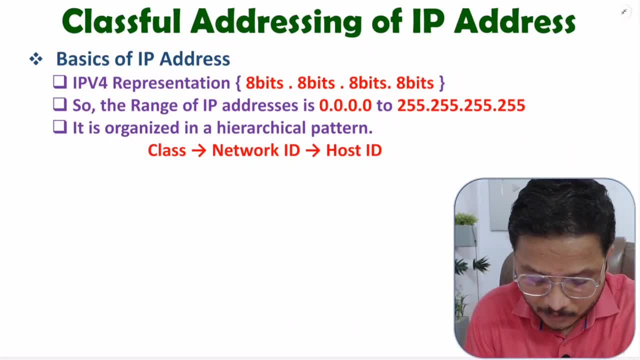 range is there. So IPv4 IP address range that is there as per 0.0.0.0 to 255.255.255.. And see IP addresses. that is organized as per hierarchical structure. In my previous video also I have discussed 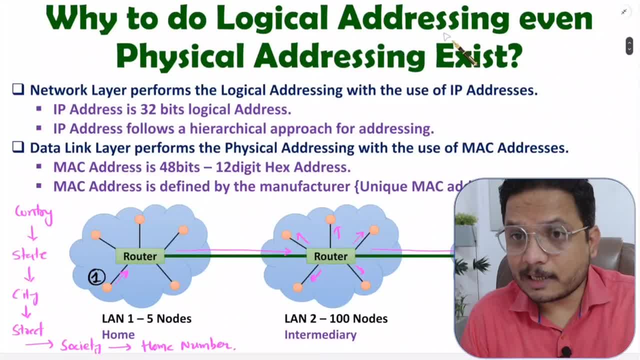 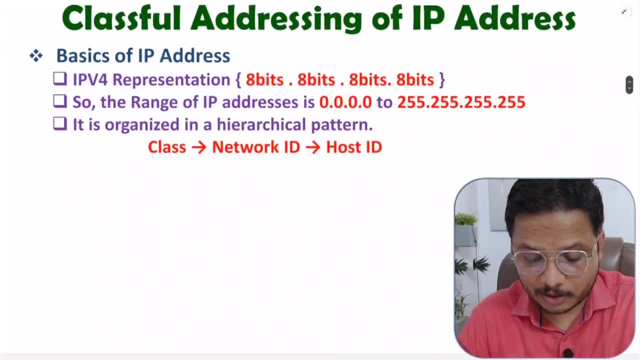 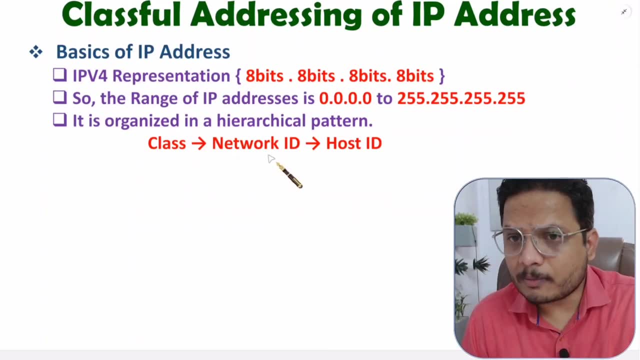 like: why do we need to have logical addressing? The reason is: logical addressing is done with the use of IP address. It is having hierarchical structure. Like you see, it is defined as per class And after class you need to go for network ID. From network ID you need to go for host ID. So 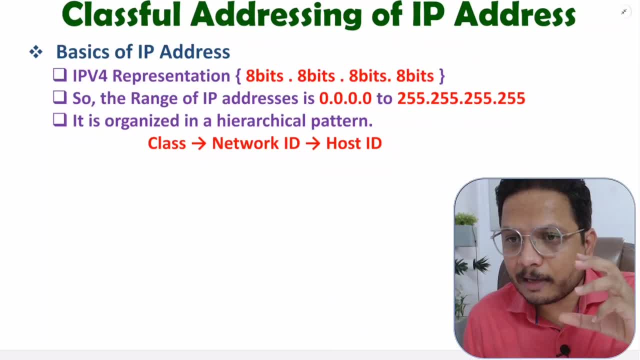 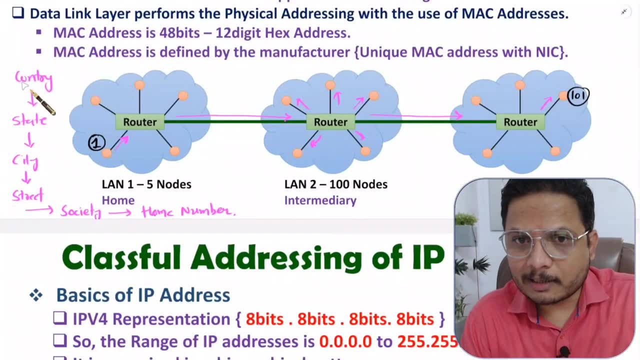 whenever routing happens, at that time it will be having hierarchical structure, Like when we say we want to send something with respect to country, then after country there will be state, then city, then street, then society and then your home number will come. 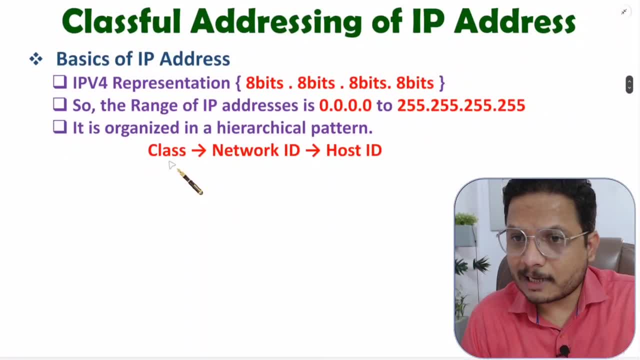 Right. So basically in IP address there is a hierarchy, Like there will be one class After class. you will have to see what is network ID. After network ID you will have to see how host ID is there, Right? 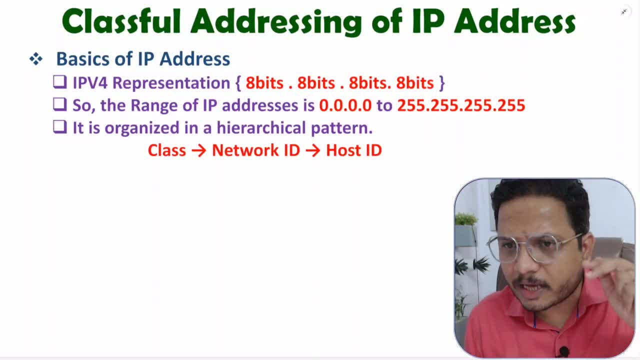 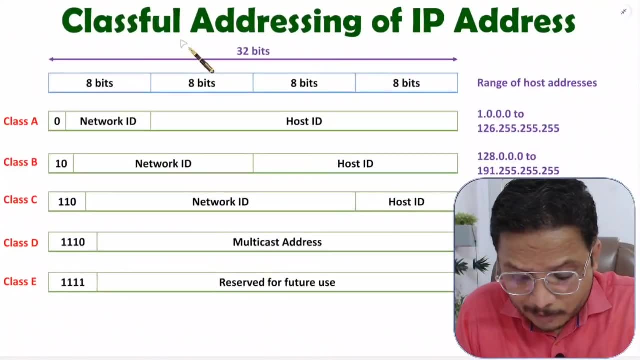 So that is how hierarchical structure is there, So that hierarchical structure that I'm going to explain you by complete details, along with classes. So let us see classful addressing of IP addresses. So in classful addressing of IP addresses, basically we are having five classes: Class, 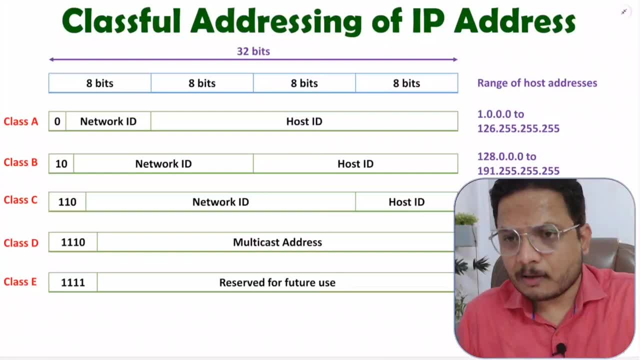 A, class B, class C, class D and class C. First of all, I'll explain you how we can remember those classes. The reason is you will have to understand that with respect to how IPs are there, As well as in examination. 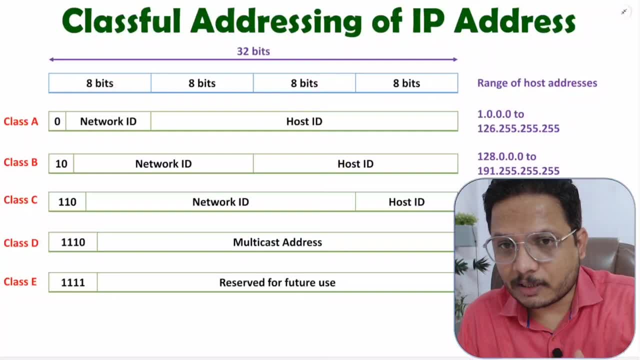 you will have to remember, like how those IPs are organized. So it is quite simple. You see, total bits are 32.. And that is there as per one octave, dot one octave, dot, one octave, dot, one octave. In total, four octaves are there Right. So here you can see that the 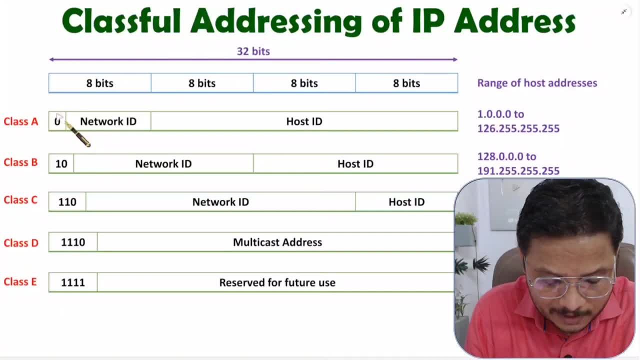 first octaves are there. So here, with class A, first bit will be zero. With class B, first two bits, that will be one zero. With class C, first three bits, that will be one one zero. With class D, first four bits, that will be one one one zero. And with class E, first. 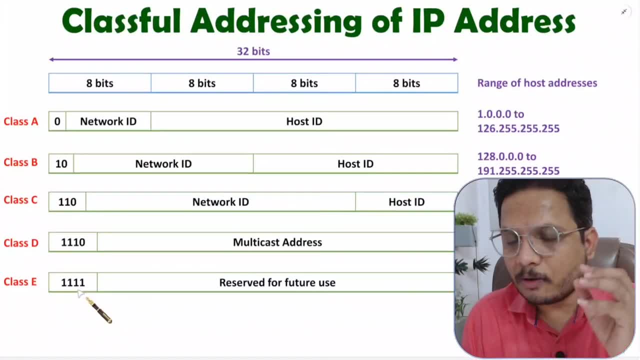 four bits, that is one, one, one, one. See, that is how bit pattern is there. After that you will have to remember few basic things only, Like network ID with class A, that is there up to first octave. With class B, network ID is there up to second octave. With class C, network ID is there. 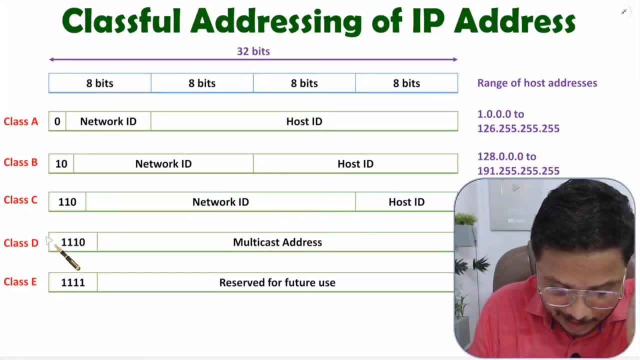 up to third octave, And with class D and class E we are not having network ID and host ID Right. With class D, we are having multicast address And class E that is reserved for future as well as for research. Now you need to understand this. also With class A, how? 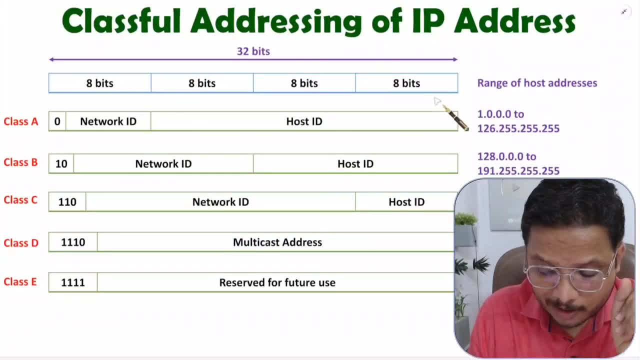 many host IDs are there. They are there for three octaves. So last three octaves that is there, with host ID for class A, With class B, last two octaves that is there for host ID And with class C last. 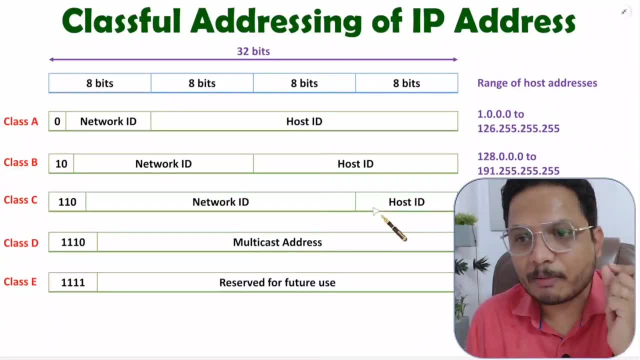 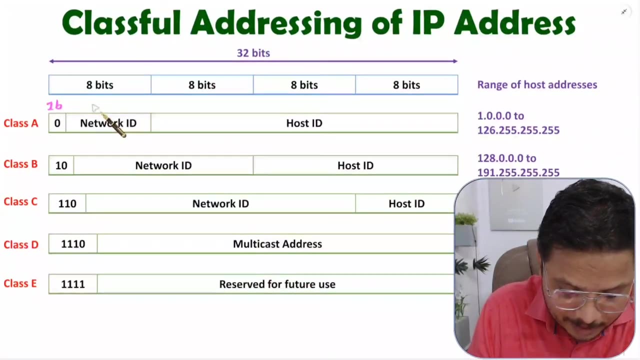 one octave. that is there for host ID. See, this is how you can remember all the classes. Now let us discuss about how many basics are there with all the classes. Like you see here, with class A, first bit, first bit that is zero, And then network ID is having three. 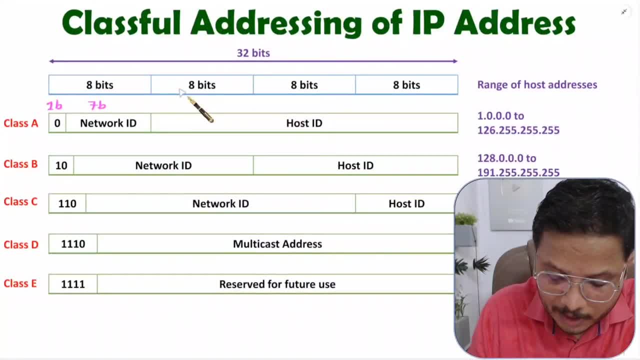 seven bits and then host id. that will be having three octaves means 24 bits. right, with class b. first two bits, first two bits, that is one zero, and then up to second octave. network id is there. so two octave is having 16 bits. so 16 minus 2, that will be 14 bits with network id. 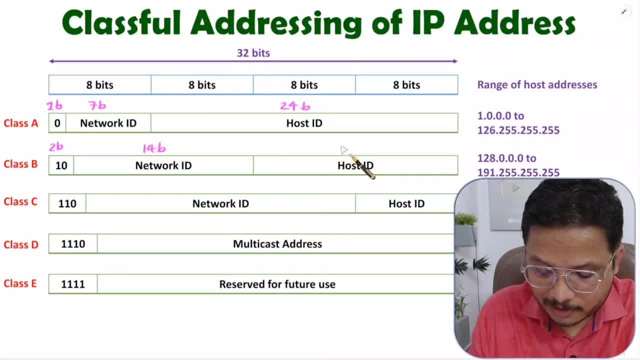 with class b and host id is having two octaves, means 16 bits. with class c, first three bits, that is 1, 1, 0, then up to third octave, network id is there, so 24 minus 3 that will be 21 bits of. 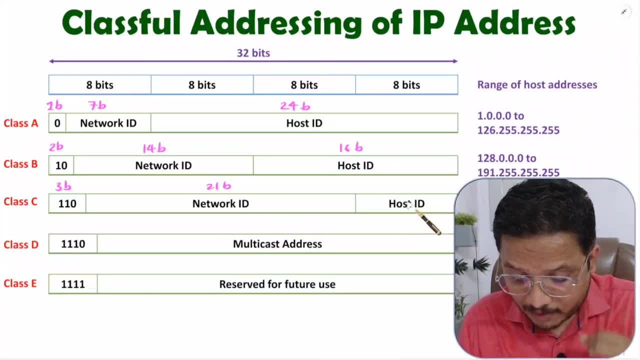 network id, right, and host id. that is having one octave only. so 8 bits with class d, in total 32 bits are there. out of that 4 bits, that is 1, 1, 1, 0. those are first 4 bits and then multicast address. that will be having how many bits? 32 minus 4. 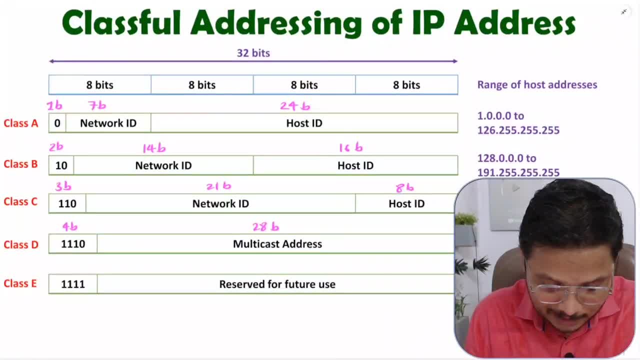 that is 28 bits right. and similarly with class e. first 4 bits are 1 1 1 1 right and reserved bits for future. that is having size of 28 bits. see, this is how number of bits that you can understand. now there are few basic things that i would like to discuss about. each and every class right, like 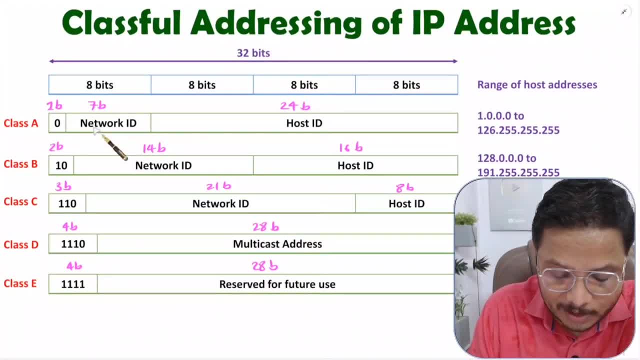 when you talk about class a, then network id is having how much size. you see seven bits, right, and it will be always zero. so what should be the range of class a? then all seven zeros, after that zero, then all seven ones. so all zero means zero and zero, and then seven ones means 127. so class a 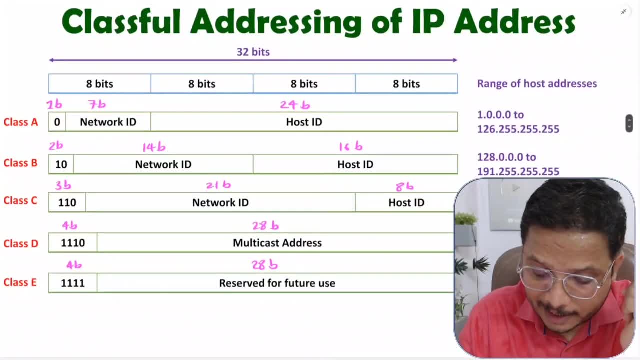 that is having first octave. that represents what network id right and it is having minimum value one. why the reason is: all zeros and what is relationship between the class are resolved. that is not given to any network right and all ones of network id. that is also. 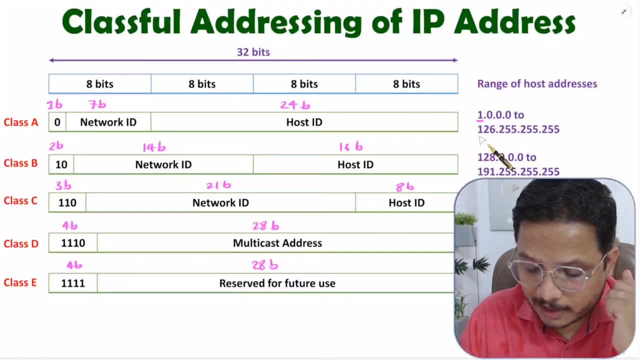 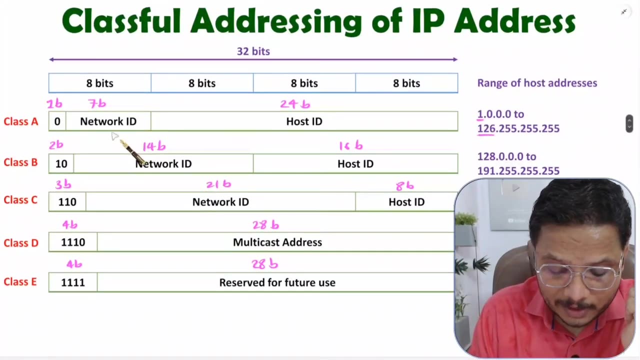 resolved. that is also not given to anyone. so instead of range that is there from 0 to 127, it is there from 1 to 126, right, 127. that is resolved. and by this pink color i am showing you this octave as per network id. you see, network id is there for first octave, so first octave, that is. 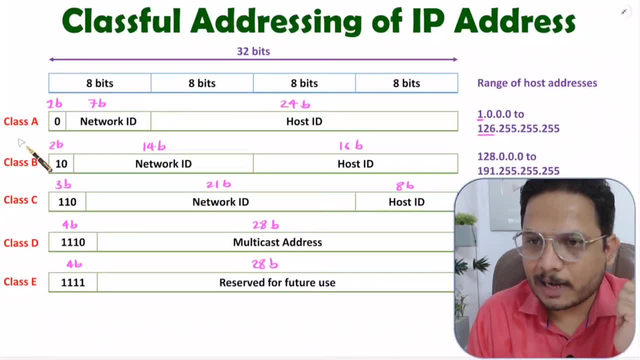 there from 1 to 126 with class a right. in some books it may be written as per 127, but remember 127, that is resolved. that is not given to any network id right now when you say how many network ids are there with class a. so this is how you should remember: see 2 to the power, 7 minus 2. so 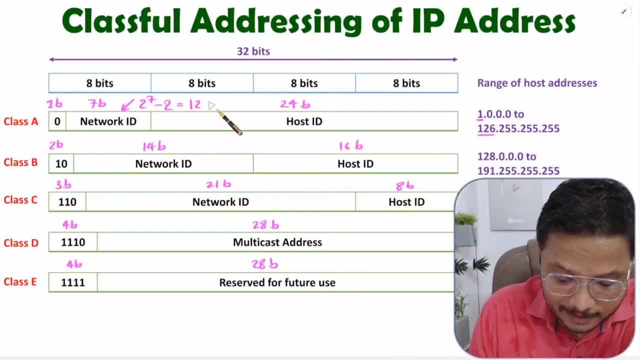 that is 120, 126, right 2 to the power 7, that is 128 minus 2, that is 126. so with class a total network ids those are 126. now let us see what is there with class b. see in class b first two bits, that is one zero. so obviously with this network id range will be from: 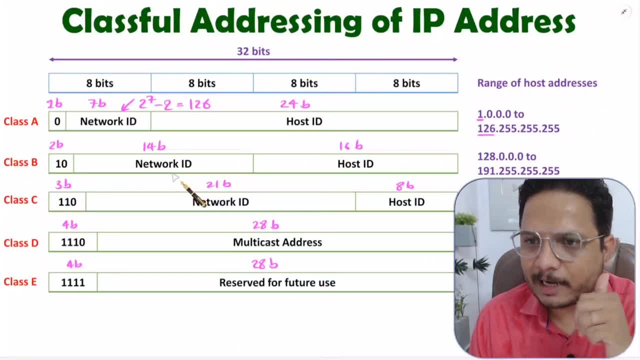 14 zeros to 14 ones, right? i'm not writing it over here, you just understand that, right? and as if one zero and after that all zeros are there, then obviously, what is that value? for first octave one, and then seven zeros, that will be 128. so first octave, that is 128, but remember, with class b, second, 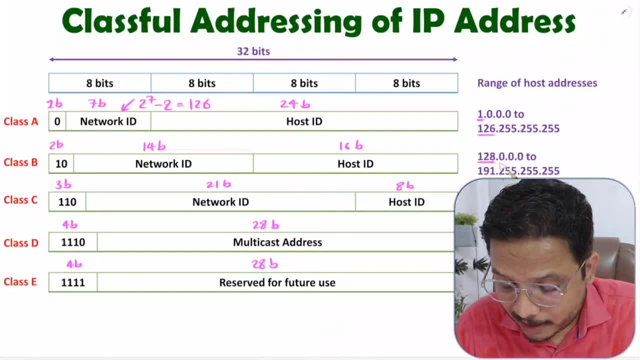 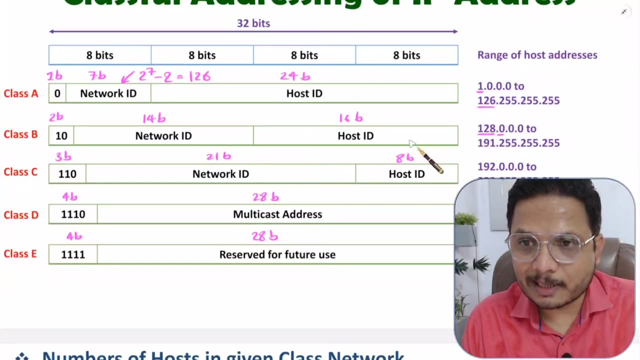 octave. that is also belong to network id, so i am just marking it over here. so initial value, that will be having range from 128.0.0.0 right, and final value will be there from first two bits, one zero, and then all ones are there. what it means it will be 191. 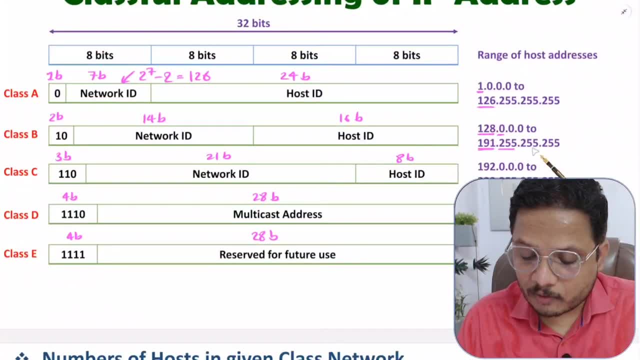 then 255, right, and then dot, 255, dot, 255. but you see this 255 that belongs to this 255, that belongs to host id, right? so here, as if question is: how many network id is there with class b? then you can say: it is 2 to the power 14, right, it is 2 to the power 14. now with class c. 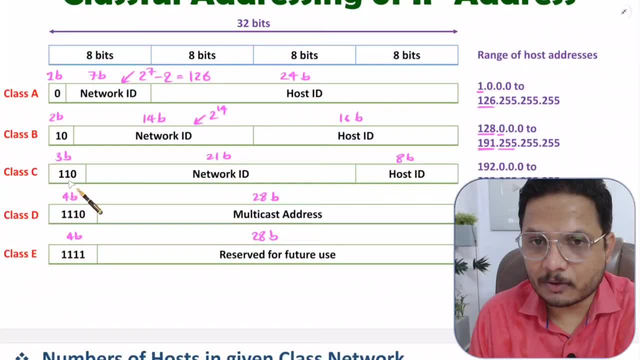 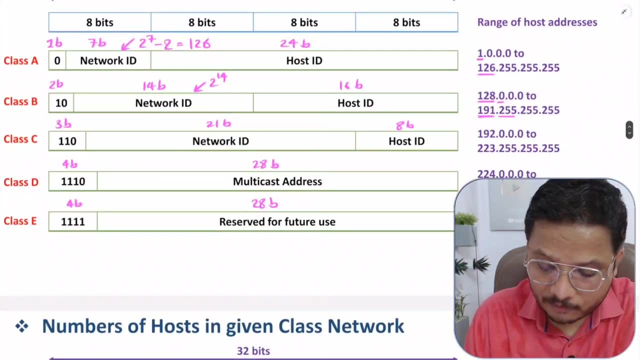 if you observe first three bits, that is one, one zero. so obviously network id is there up to third octave. so based on that you can say: based on that first three octaves, that belongs to network id and last octave that belongs to host id, right, so here what will be the range? 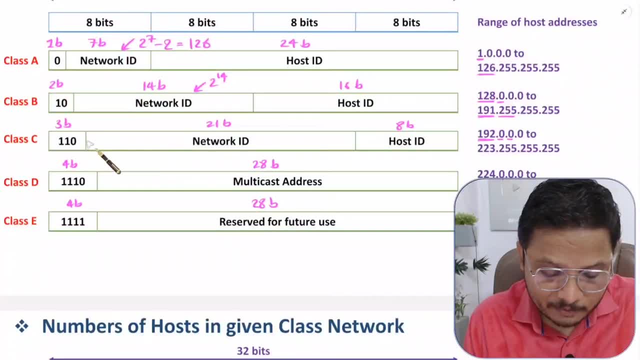 see double one zero and then five zeros are there with first octave, so that is 192 right, and then zero dot zero, see this: three octaves, that belongs to network id over here and last zero that is there with respect to host id right, and it is ranging from one one zero to all ones. 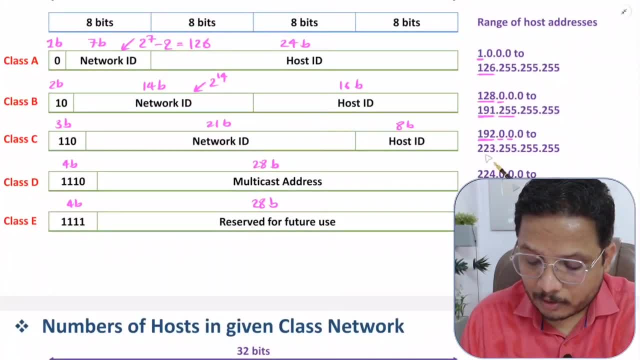 right up to all ones. it is ranging, so that will be two, two, three, dot 255, dot 255 that belongs to network id and last 255 that belongs to host id. so obviously here how many host ids are possible with given network: two to the power, eight right now with class d. 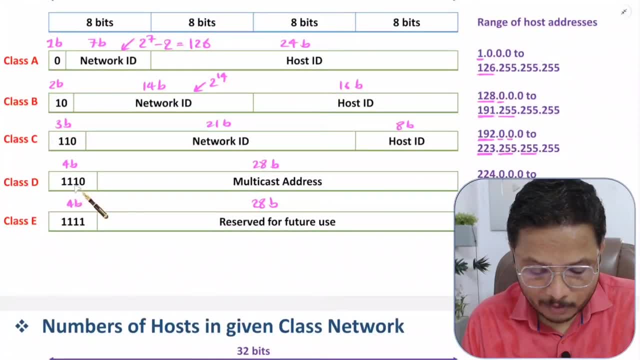 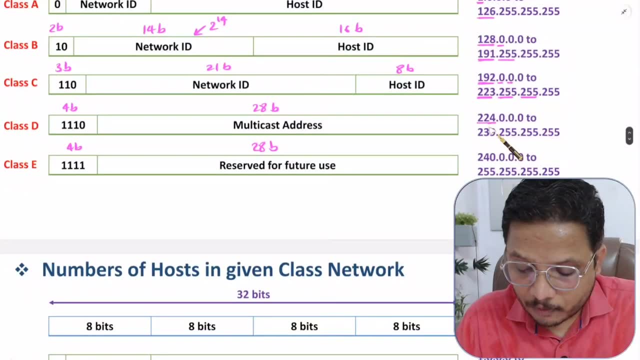 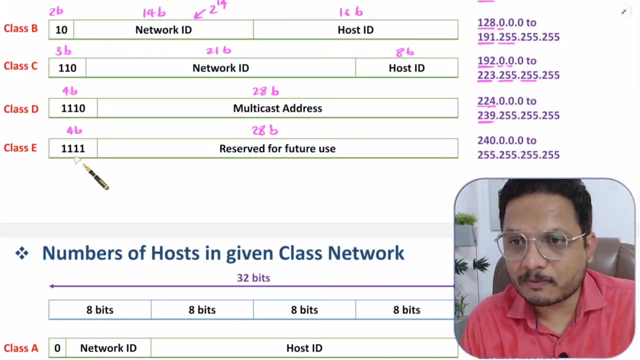 with class d, first four bits, that is fixed one one, one zero right and then multicast address bits will be there. it is having range from 224 to 239. and here with class e, it is having first four bits, that is one one one, so it will be having range from 240 to 255. now i am not going to write all. 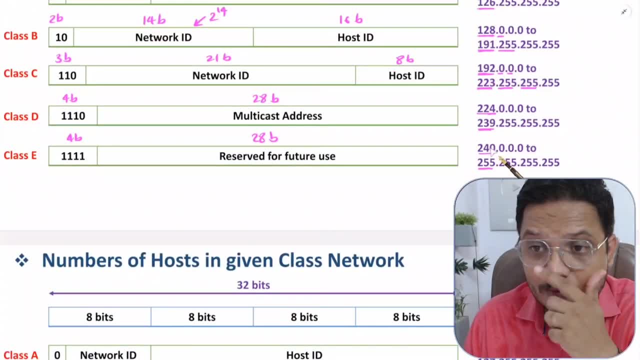 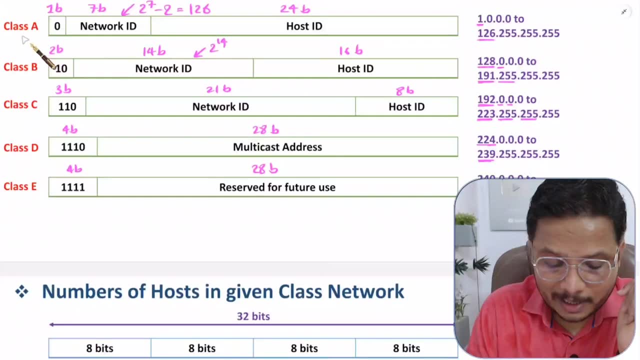 the network ips over here with respect to bits. why? the reason is: what i want is you just remember this? you just remember this ip addresses with respect to class a, b, c, d, e. see here, simply, this is how you can remember: for class a, it ranges from 1 to 127. in some books it is written up to 127, but 127 is. 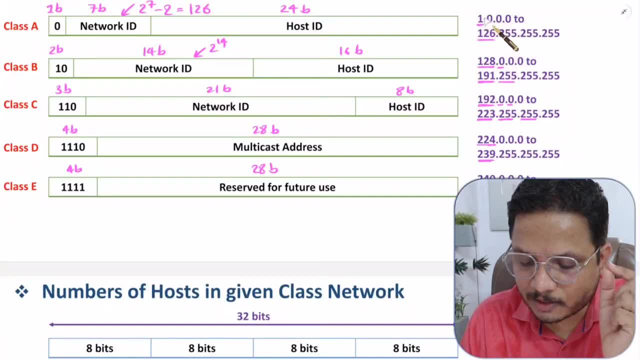 resolved. so with class a, 1 to 127, this first first octave, that will tells everything. second octave will be 128 to 191. third of then, class b is having range from 128 to 191. so this is how you can remember. for class a, this first octave is having 192 to 223. with class d, 224 to 239 with class e 242. 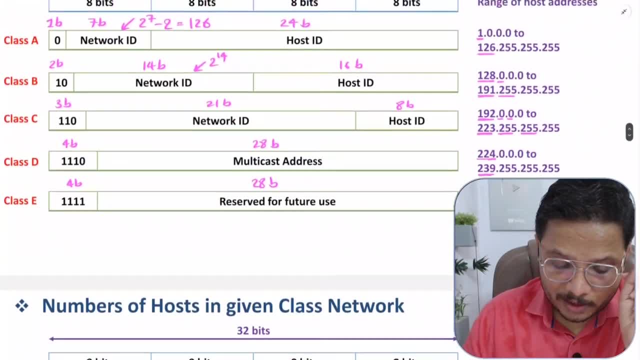 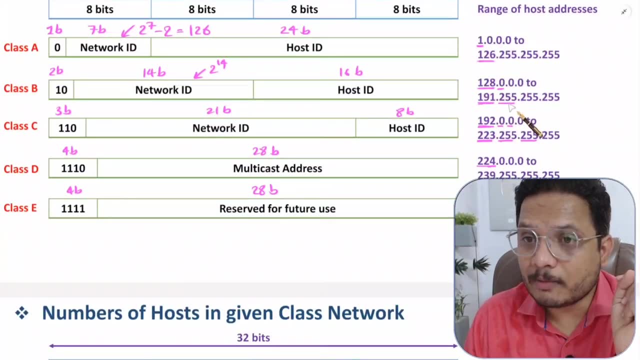 255, that is about first octave and you should know with class a, first octave only belongs to network id. with class b- first and second octave- that belongs to network id. with class c- first, second and third octave- that belongs to network ip. network id, right, or you can say network ip. 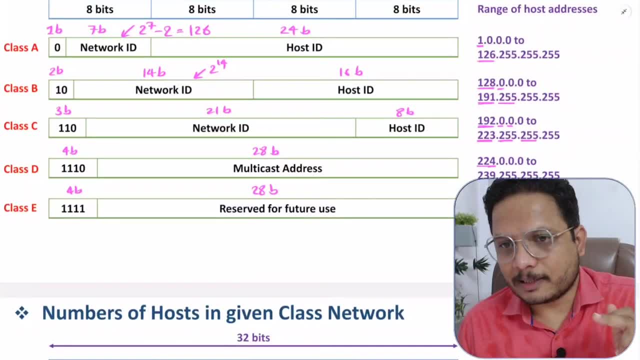 here. see, this is how we can remember all the classes right and here. this is what you will have to remember. the reason is as, being a computer science engineer, you will be finding many equations in many ways, so it is not like you will be calculating all those things as per this format. 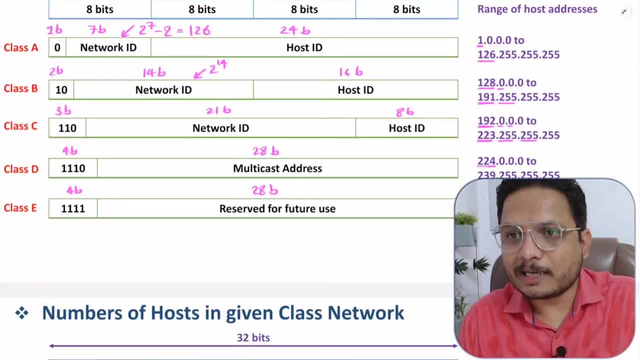 right directly. you should know, like, if it is having first octave, that is there in between one to 127, then you can say it is there with respect to class a. if it is there in between 128 to 191, you can say it is there with respect to class b. if it is there in between one to 127. 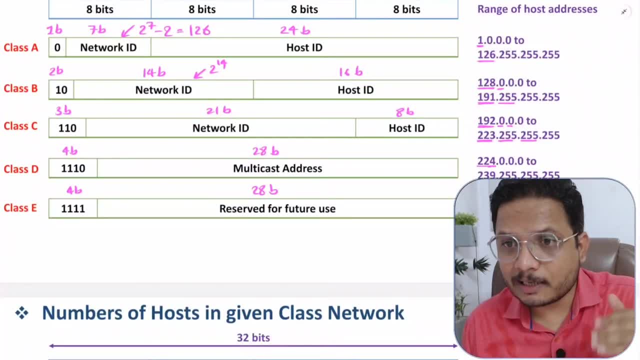 192 to 223, then it is there with respect to class c. if it is there in between 224 to 239, then it is there with respect to class d. if it is there from 240 to 255, then it is there with respect to class. 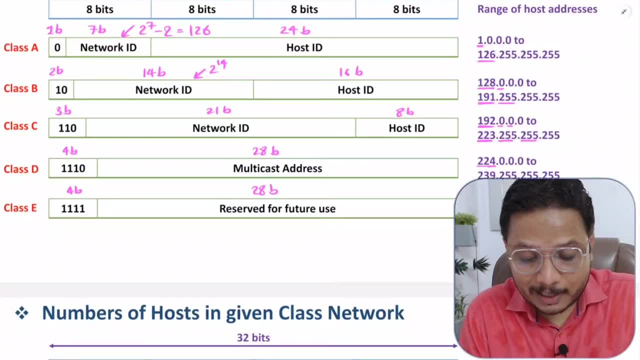 e- that is how you should remember and see- with class a, first octave that belongs to network id or network ip. with class b, first and second octave that belongs to network id or network ip. and with class c- first, second and third octave that belongs to network ip. this is how you will. 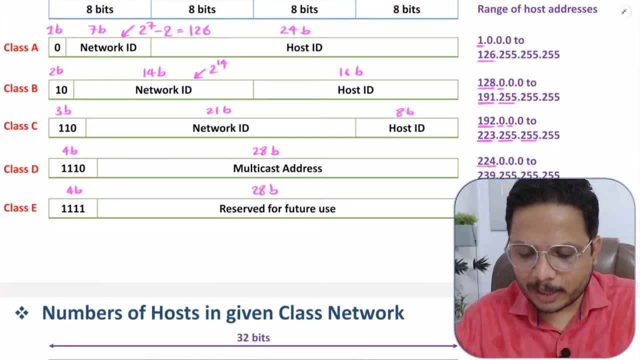 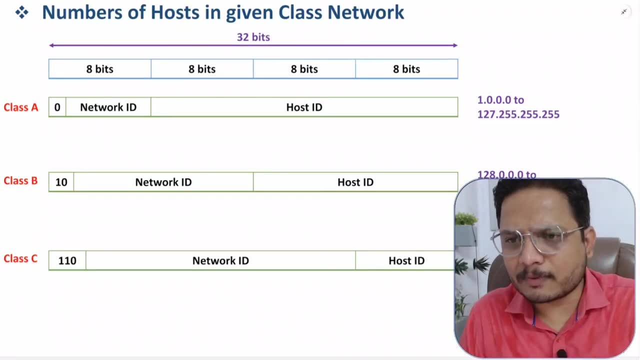 have to remember the things. now, very interesting part that i'm going to explain you now. so in that i'll explain you how many number of hosts that is there in given class of network, as well as two very interesting things that i'm going to explain you. first is what is network ip and second is what 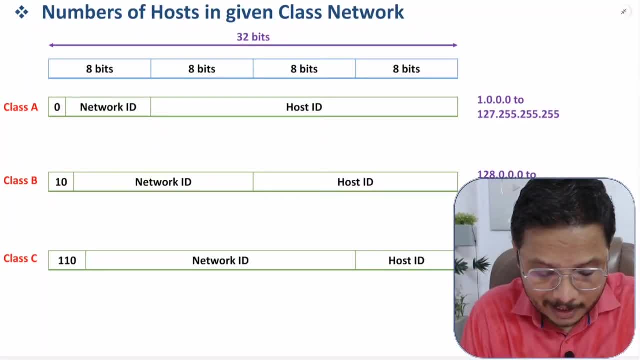 is broadcast ip, right. so with class a we have seen first bit will be zero and second is broadcast ip zero and it is having ip address range from 1.0.0.0 to 127.255.255.255. right, but when it comes to 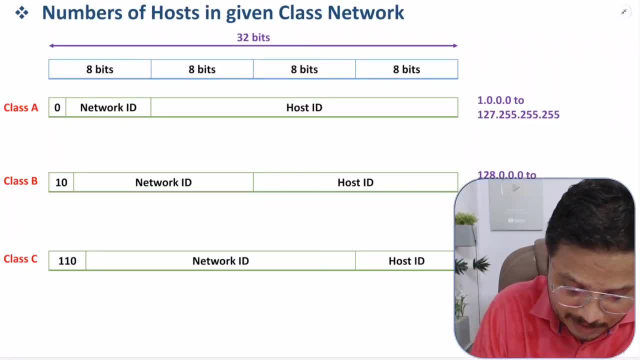 network ip. when it comes to network ip, then there are few basic things that you should know in network ip. in network ip, first, first byte, or you can say first, octave, that belongs to that belongs to network id, right? so here let me say, let me say it is 91, right. so first 91 that you'll have to write, then dot, zero, dot, zero, dot, zero. see. 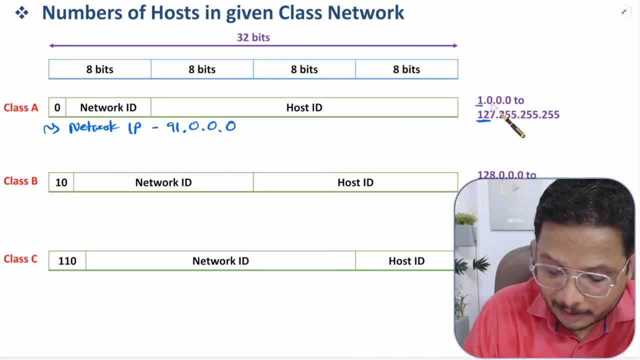 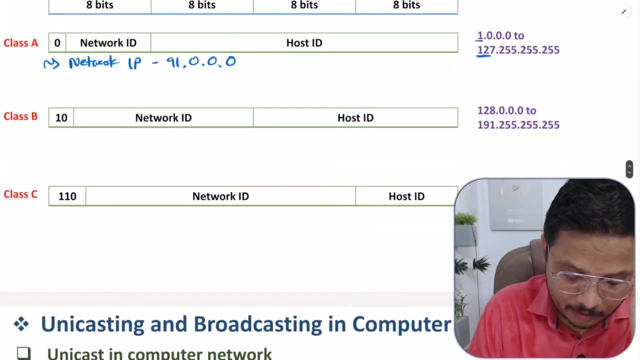 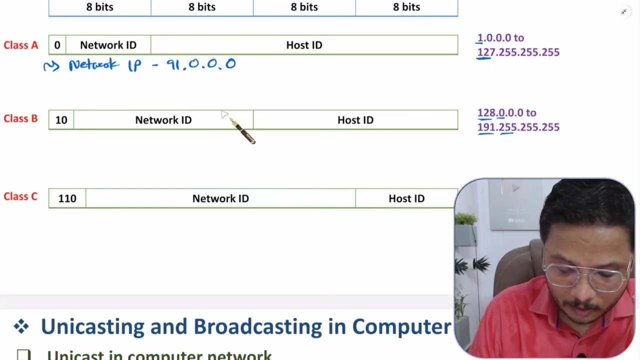 this zero dot, zero dot, zero right that you will have to keep for network ip. so every network is having network ip right. so see network id that is been defined by first, two, first octave right with class b, with class b, first, two octaves right. that is there for network id right. so as if i say i want to have one network ip, 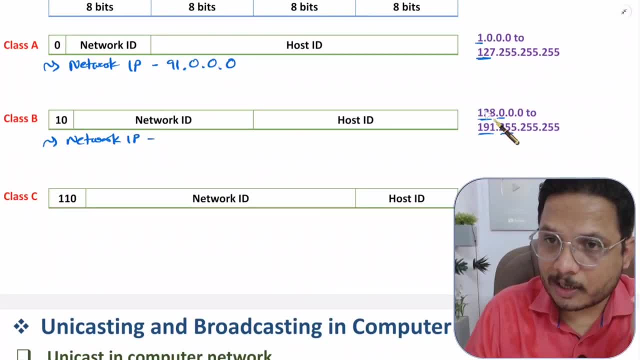 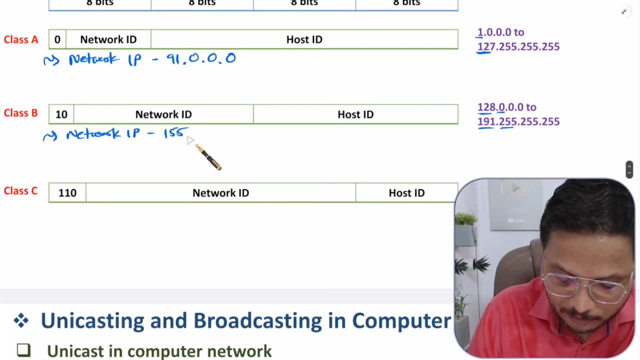 for class b, then first octave, that should be there in between 128 to 191, right? so let us say it is 155. so 155 dot 4. see, this is what network id for class b. then dot zero, dot zero that you'll have to. 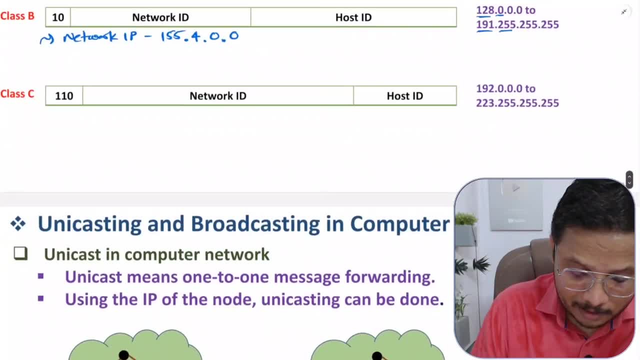 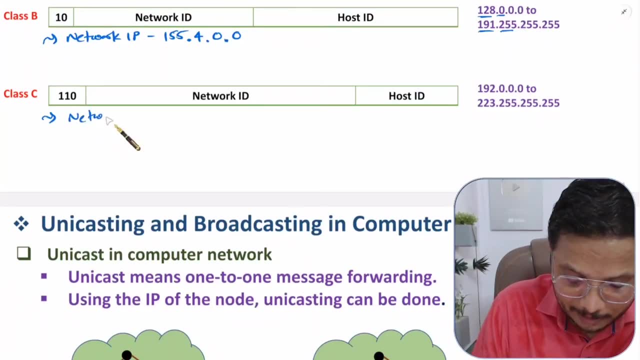 network IP, like with class C? with class C, what is the range? 192 to 223. so when you talk about network IP, let us say one example- then you will have to take three octaves for network ID. so you see this, three octaves, right, that belongs to, that belongs to network ID. so here in network ID, you 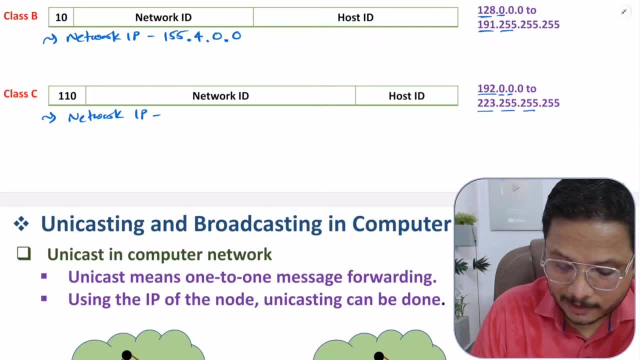 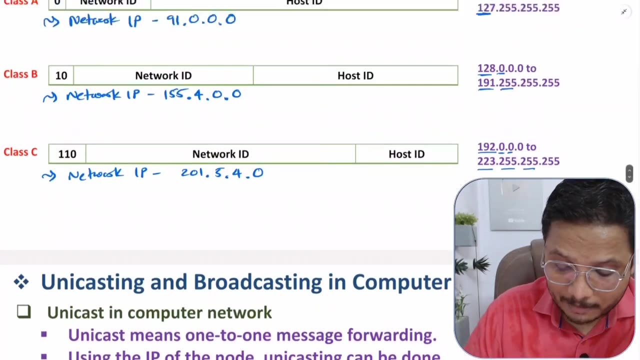 can have in between 192 to 223. so let us say I am taking 201, then dot 5, then dot 4. so this is what network ID, but dot 0, that represents network IP, right? so that is how network IP will be there. so 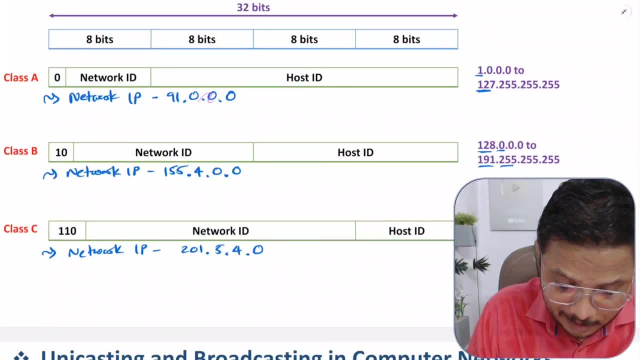 remember here: with class A, last three bits, that should be 0 for network IP. with class B, last two octaves, that should be 0 for network IP. so that is how network IP will be there. so remember here 0. and with class C, last one octave, that should be 0, right, so that is how network IP will be there. 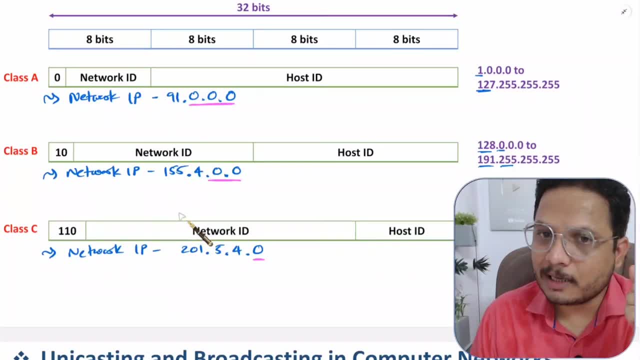 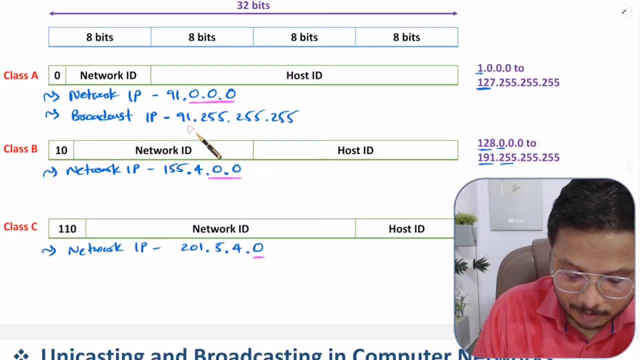 255 dot, 255, dot, 255. right, see, this is what broadcast IP for this given network, right? when you say class B with that, as if you wanted to have broadcast IP, then what is that broadcast IP? this 155 dot 4, that will be as it is. then last two, that should be 255 dot 255, right that? 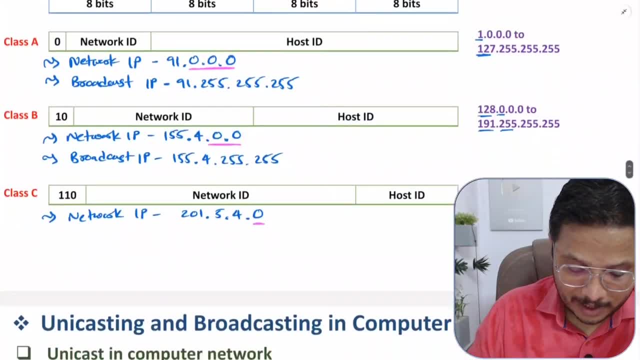 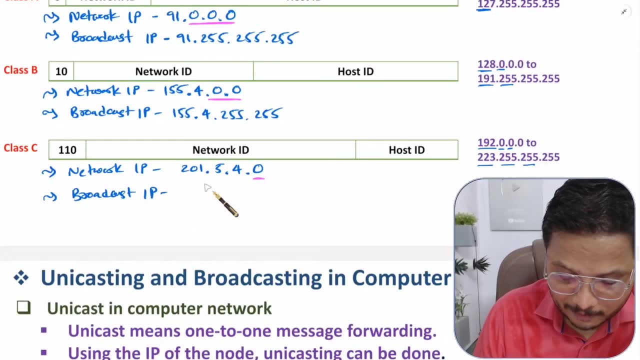 will be broadcast IP of this given network. when it comes to class C, then what is a broadcast Broadcast IP for this? that will be: this will be as it is for network ID. it will be as it is right: 201.5.4, but last should be 255. 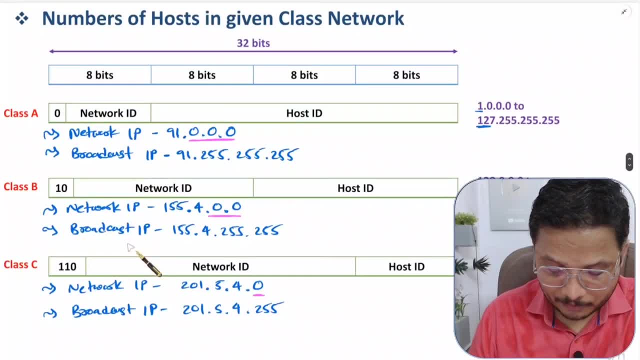 So see network IP and broadcast IP. that cannot be given to host. remember this, as if with class A, last three octaves are zero, then it is network IP. if last three octaves are 255, then that is broadcast IP. right with class B, if last two octaves are zero, that is network. 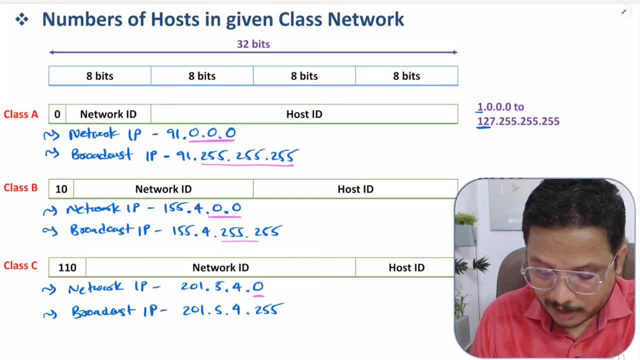 IP with class B. if last two octaves are 255, then that will be broadcast IP with class C. if last octave that is zero, then that is network IP with class C. if last octave that is 255, then that will be broadcast IP right Now. 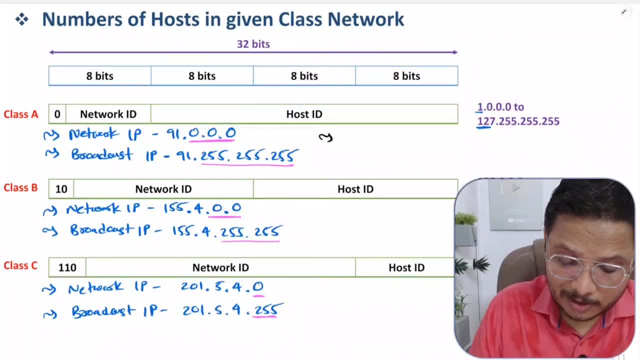 Now, Now I'll explain you how many host that can be there with given network IP. So number of host, number of host with class A that can be based on this many bits, right? So here we are having three octaves, So two to the power. three octaves is having how many bits? 24, so two to the power, 24 host. 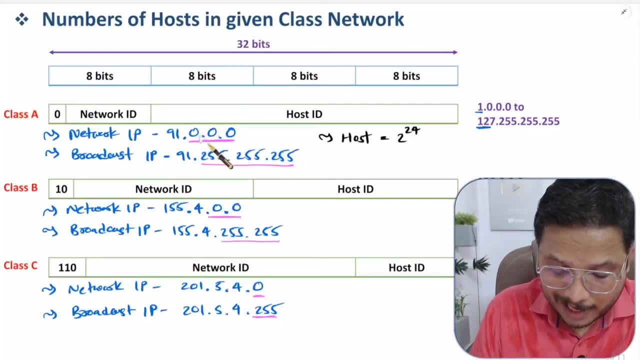 but see, out of two to the power 24, two IPs are reserved. one is for network IP and second is for broadcast IP, right? So minus two that you'll have to do, that will be number of host in given network IP right Now. as if question is: how many host? how many host are there in class B, then in class B? 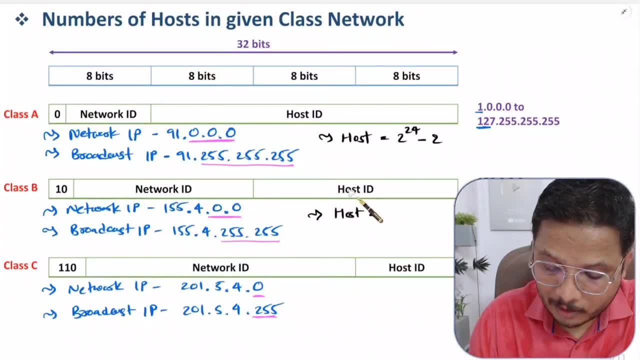 how many host are possible. So host is having how many octaves? two octaves with class B, so two octaves means two to the power. 16 hosts will be there, but out of that two IPs- that is reserved for network IP and broadcast IP. 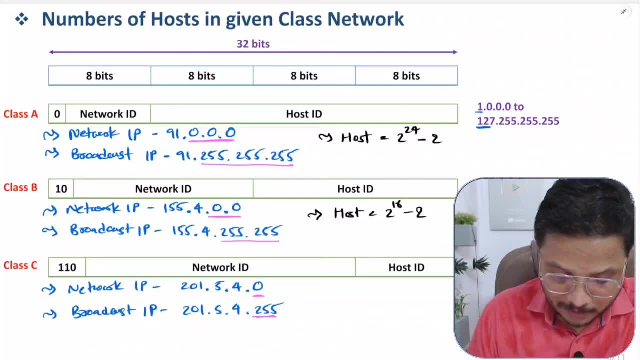 So two to the power 16 minus two Right. when it comes to class C, how many host are there? So number of host, that is based on one octave of host ID over here. So that will be two to the power eight minus two right. 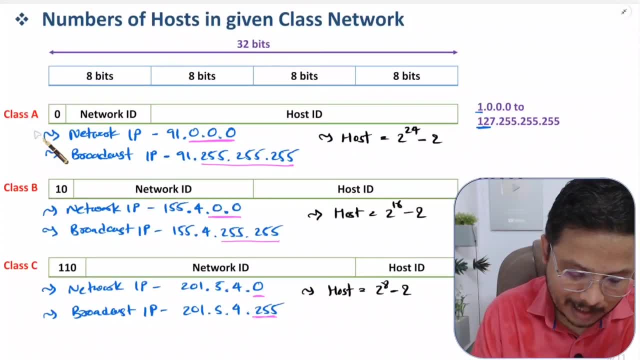 So that is how number of host that we can identify for given class IP, like one network is having how many host that can be calculated as per this. So you should be having fair enough idea about for any given network. There will be one network IP and there will be one broadcast IP and those two IP addresses. 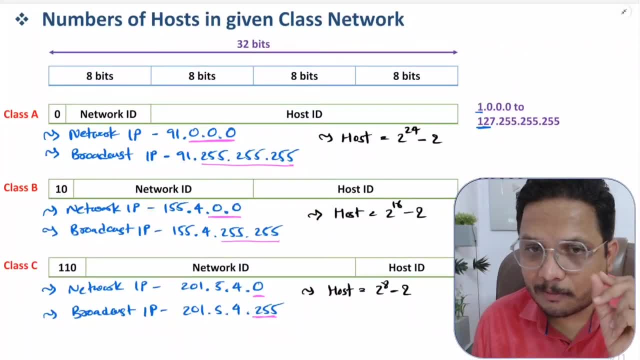 cannot be given to host right. So how many host will be there? So with class A, we are having three octaves for host ID, so two to the power, 24 minus two. With class B, with given network, two octaves are there with host ID, so two to the power. 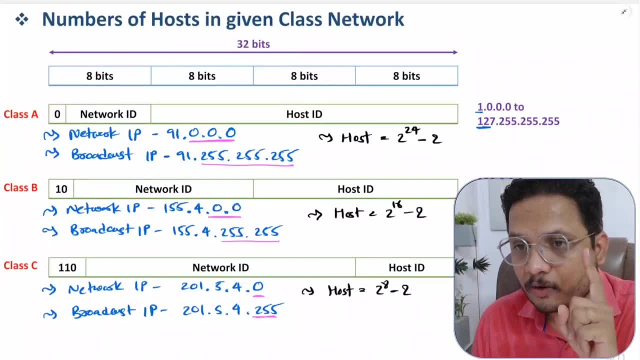 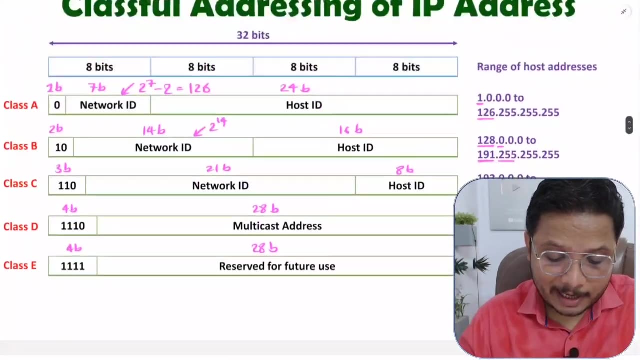 16 minus two. With class C, we are having one octave for host, so two to the power, eight minus two, Right? So what is coming? based on network IP and broadcast IP, right? So now I think you are having exact clarity regarding how classes are there, right? 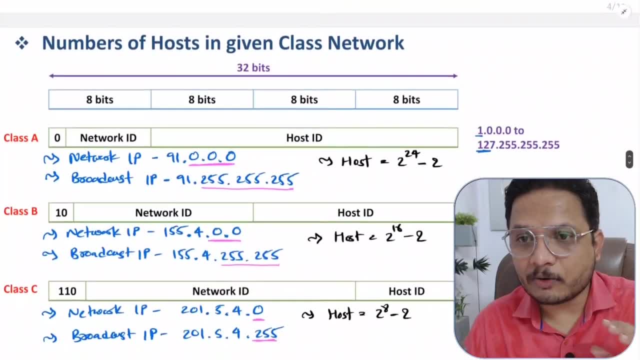 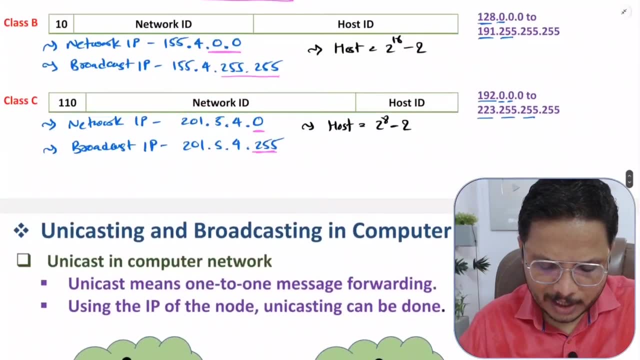 So this is how classes are there right? These are the basics that you need to understand, right, And based on that, now I'll give you two very practical case studies like how we can have unicasting and broadcasting. So in unicasting, first of all you should be having basic understanding like what is unicasting? 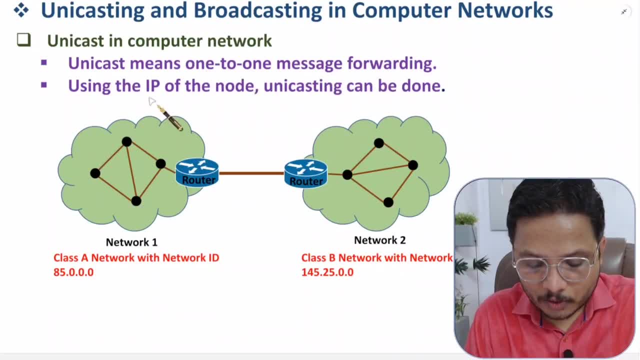 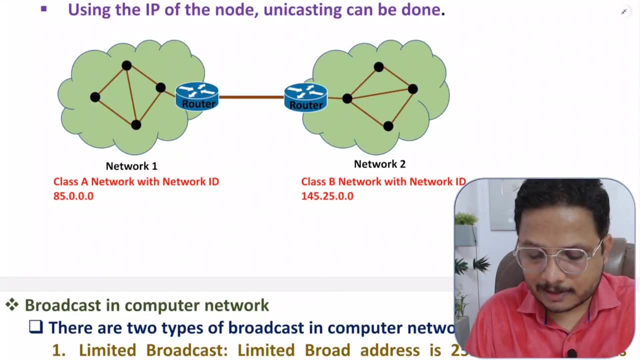 See unicast means one to one message forwarding. So using IP of node unicasting can be done. Let me take one example. like here: we are having one network and this is second network. Let us say this one network that is having one node over here and we are having second. 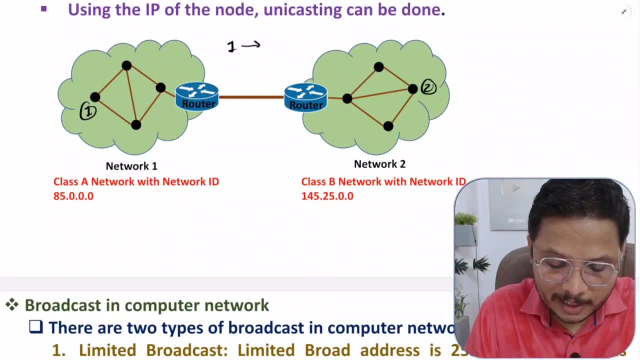 node over here and we wanted to have transmission of data from one to two. Then how this node number one will forward data to node number two. So that will be done with the usage of IP of node one. Now, what could be the IP? 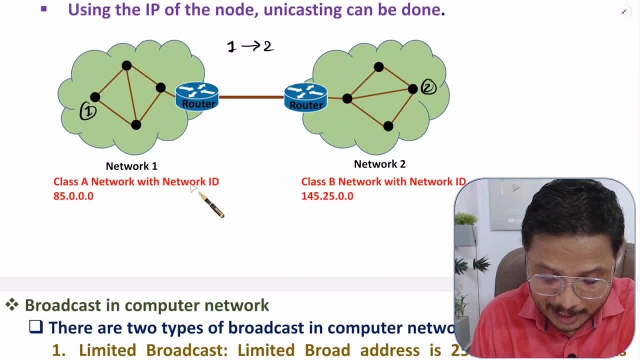 IP of node one means IP of host, So that depends on network ID. Now here I have taken example of class A, in which class A is having class A is having first octave, that represents network and last three represents last three represents host. But zero, zero, zero means this is network ID or network ID, right? 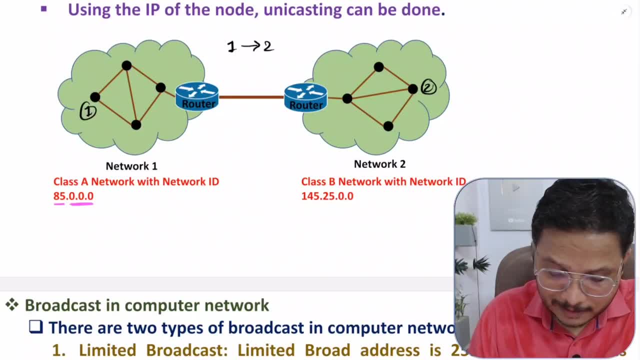 So let us say this host number one Is having IP that is 85 as per network ID. then let us say it is 5.4.1.. So that can be, that can be host ID in this given network, right with host one. 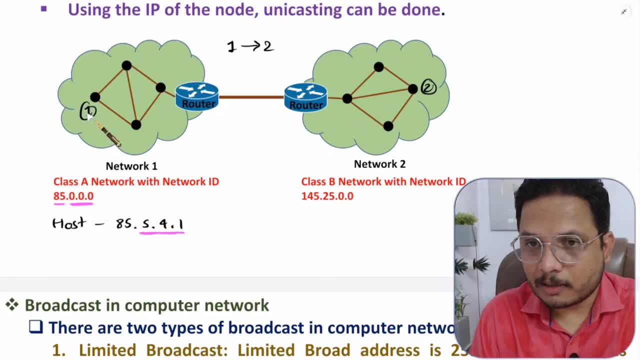 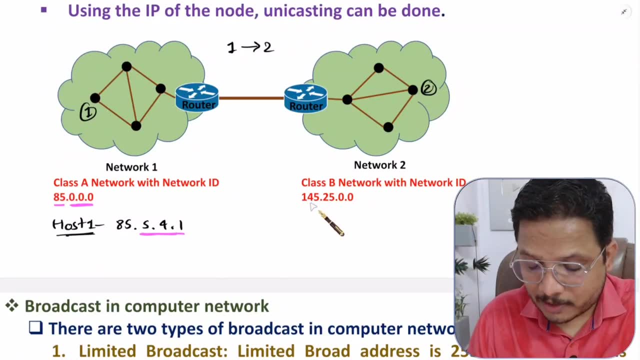 Now, similarly as this host one is having this ID with host two, it will be having ID based on: based on host two. So this is host two. This is host two. This is host two. So this is what ID is network IP of this network two. 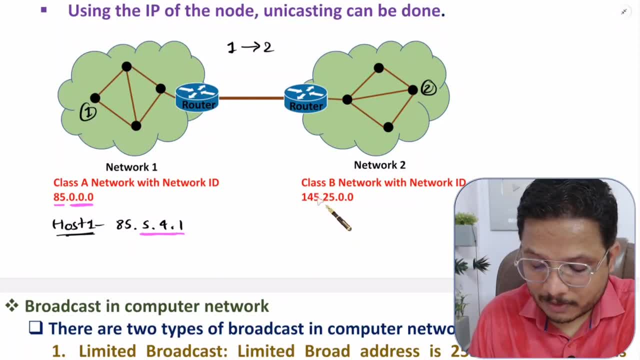 So you see, this is what class B type of this, is what class B type of network, how we can identify that. you see, first byte that is 145.. So that belongs to 128 to 192 means you can say: this is class B type of network and first, 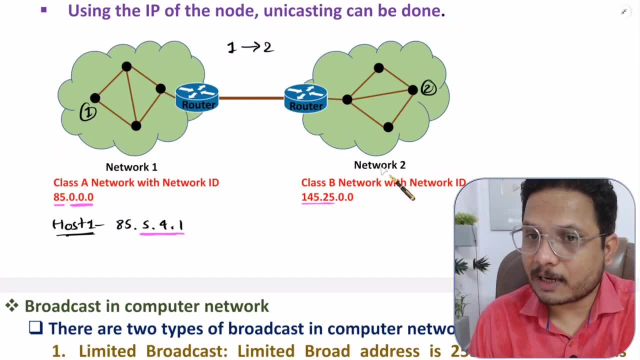 two octaves. that represents network ID. after that you see zero, zero is. that means this is network ID of given network. now with host2, what can be with host2? what can be, what can be ip? so first two bytes, that will be, as it is, 145.255, but last two octaves that can be anything like 1.4, right? 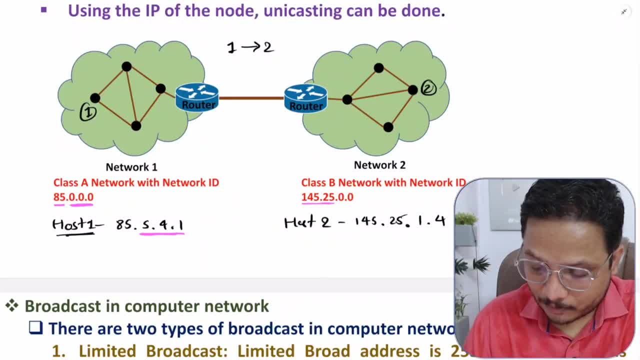 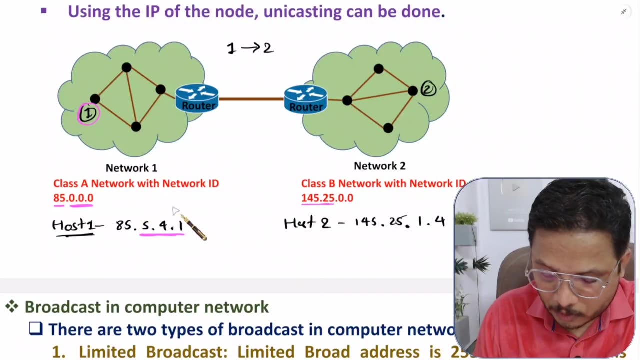 so that is how host2 ip is there now. simply, when this, when this host1 wants to forward data to this host2, then this host will be placing ip address. host1 will be placing ip address of source and destination and, based on that, with with this router, with this router, it will forward. 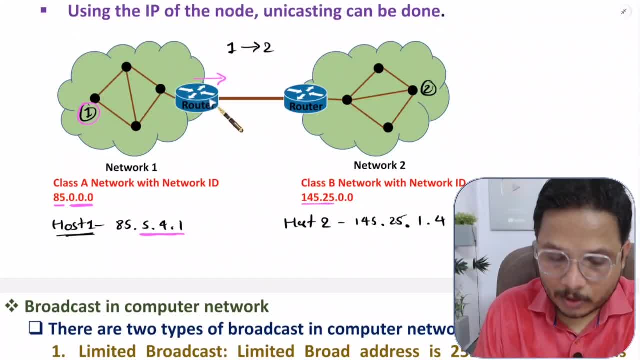 data and this router. this router belongs to network1, so it will be having network id of this and this router that belongs to class b with this network right, so that will be having this id. so first of all, it will take this message over here and after that, based on, based on: 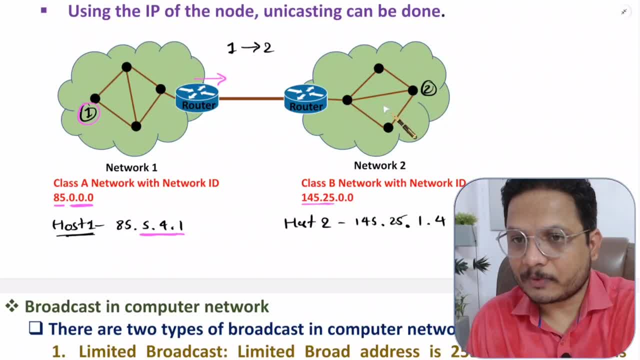 host id, it will forward it in this network right, so one-to-one unicasting. that is how it is happening. so based on network id and network based on network id means network id will define network ip right as in class. a first byte that that defines network id and based on that network ip. 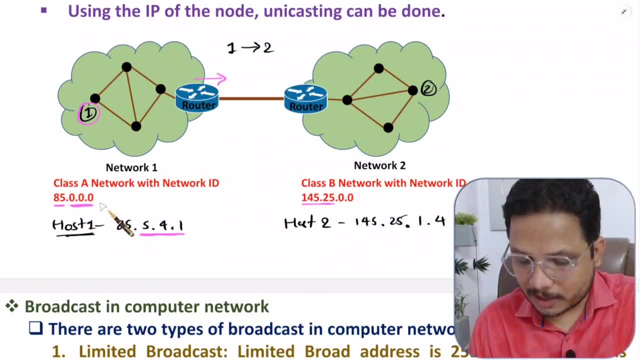 will be there in network id will be there in network id and based on that, network, ip will be IP. there will be 0.0.0 with class B. first two octaves will define network ID and based on that, network IP will be there, in which last two octaves will be. 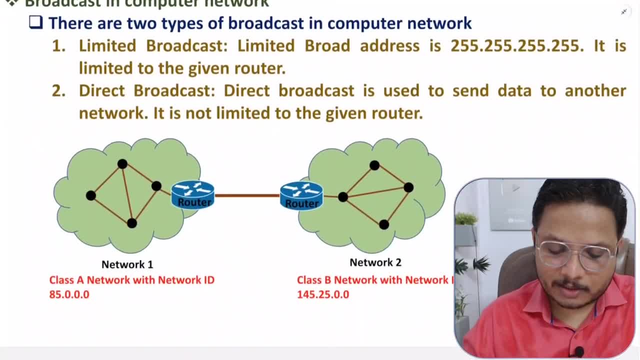 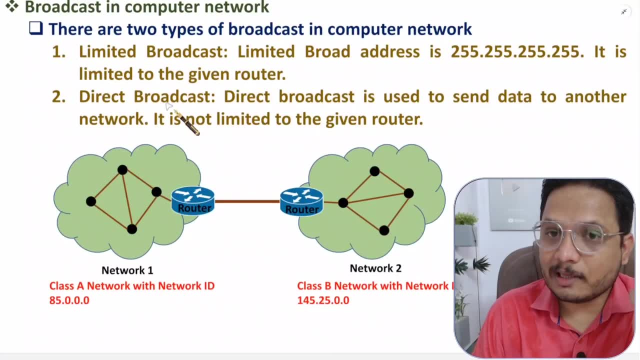 0: 0. right now let me explain you. broadcast broadcast is quite interesting. see, there are two categories of broadcast: limited and direct. so in limited broadcast, in limited broadcast, what we need to do is in limited broadcast, we can broadcasting given network, for example, as if this node, as 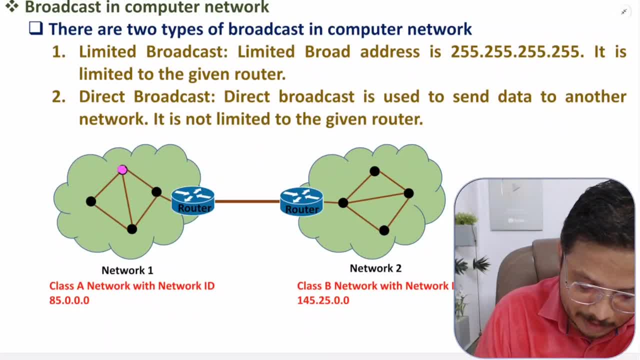 if I say this node wants to broadcast message, right, this node wants to broadcast message, then this node will have to use this IP. if this node is using 255 dot, 255, dot, 255, dot 255, then you can say this node is broadcasting message in this network. so 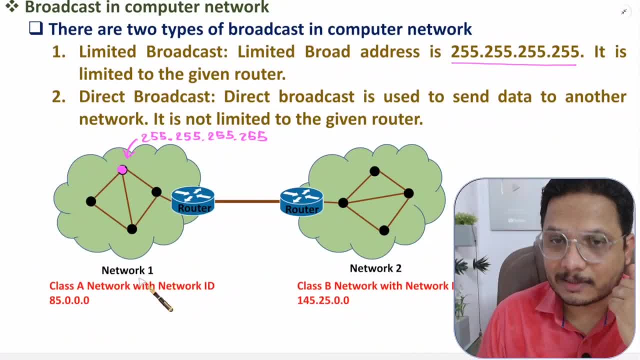 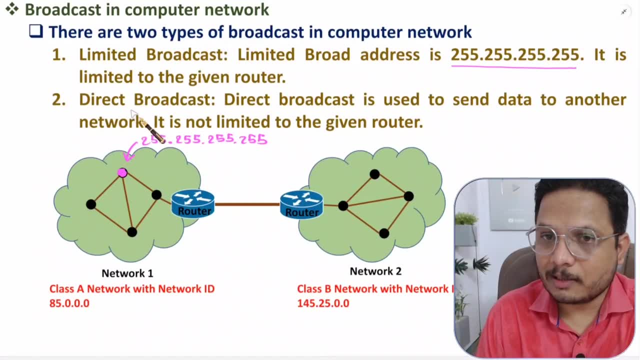 in this business we can broadcast an IP, this data, this is called process, this based on entire network, network one. it will be broadcasting message. that is, limited broadcast right now, now, as if we want to do direct broadcast, then see, direct broadcast can be done from one network to. 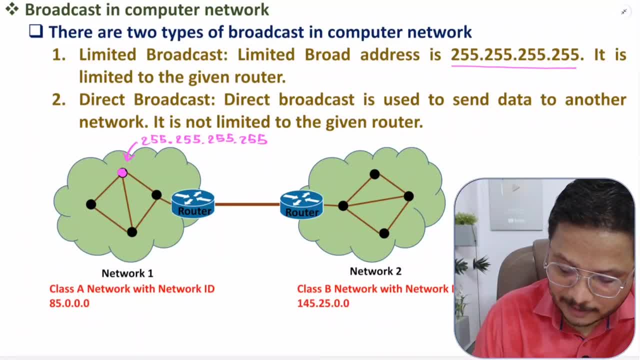 another network, for example. for example, as if i say, here we are having one node, now if this node wants to do broadcast in this network, then this node will do what this node will use- ip of this network. so as, if this node wants to broadcast message everywhere over here, right, then this node will be using which i ip of this. 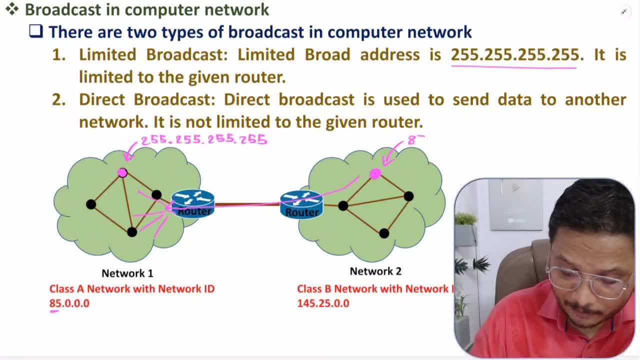 network. see first will be network id, that is 85, then dot 255.255.255. see, this is what broadcast ip for this network. so this node will be using this ip address and when it forwards this frame via this router to this router, this router will broadcast this: 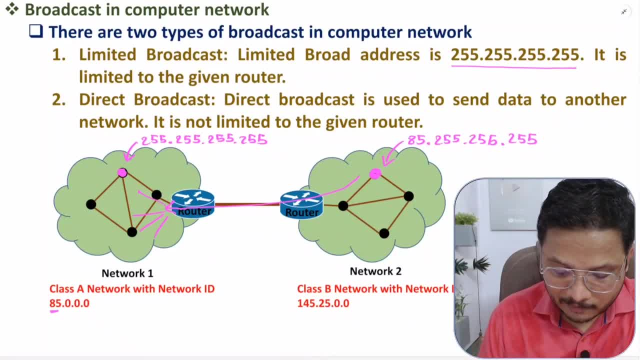 message in this internet, right? similarly, as if this node wants to broadcast message in this internet, then it will be using- see this class b type of network, in which 145.25.255.255- that ip that will be used by any of this node to broadcast message in this network. simply, this is how we are. 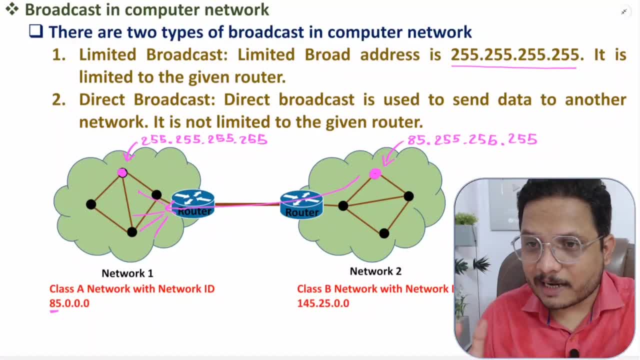 now i think you are having fair enough idea about how ip addresses are there, how classful like classful addressing is happening, right, and if still anything that you like to share, please note it down. and we are doing so much hardware, so i would like to have your support and for that, 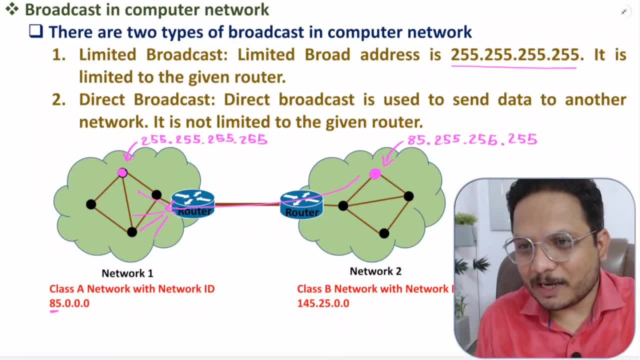 i request you to do sharing of these videos with your colleagues. definitely that will help, help us even. thank you so much for watching.